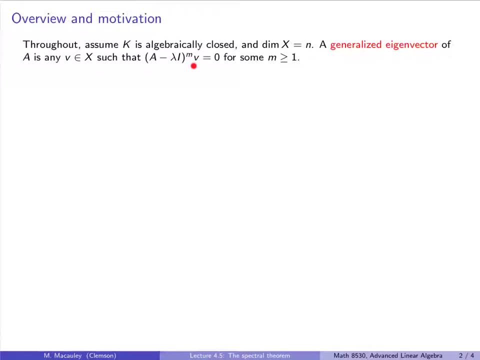 that a-lambda i to the m times v is zero for some power m. The Spectral Theorem says that for any linear map A, our underlying vector, space x, has a basis of generalized eigenvectors of A. Let's recall our running example that I have shown in several previous lectures, which 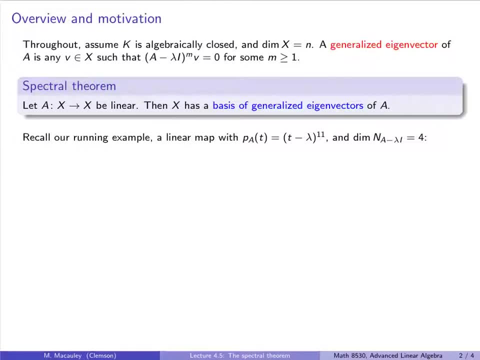 is a linear map With characteristic polynomial t-lambda to the 11,, so it has one eigenvalue with algebraic multiplicity 11, and it has four eigenvectors. In other words, the dimension of the null space of a-lambda i is four. 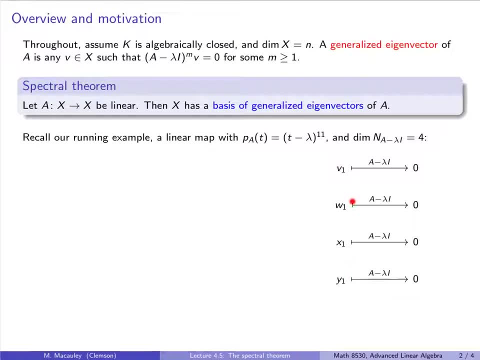 In other words, there are four linearly independent eigenvectors of A that get mapped to zero by a-lambda i. Now, what we usually want is a basis of eigenvectors of our entire space, But if we have a linear map like this and we only have four eigenvectors, we obviously 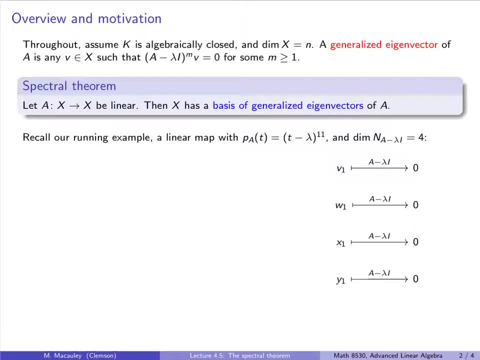 can't get that. So the idea of the Spectral Theorem is that we can at least find vectors that map on to these eigenvectors. In other words, maybe there are vectors v2,, w2, and x2 that map on to v1,, w1, and x1. 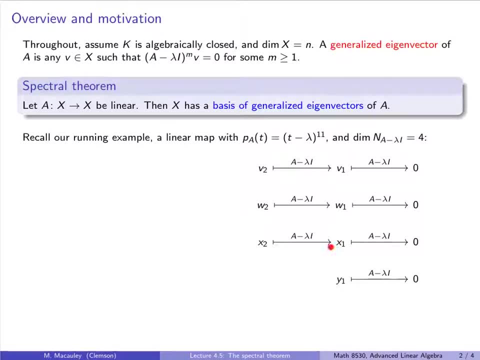 So what we want is a basis of eigenvectors of our entire space, but if we have a linear map like this, we only have four eigenvectors. we obviously can't get that, Because these are generalizing eigenvectors, because a-lambda i squared sends these things. 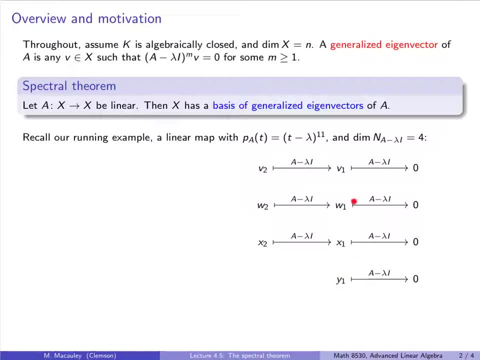 to zero. Now, if you believe that these eigenvectors are going to be independent, then this is a seven dimensional subspace And we still have an eleven dimensional subspace, So we don't have a basis. So there might be vectors v3 and w2.. 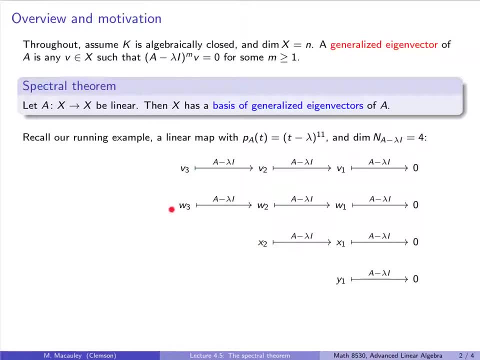 three that get mapped on to these. these are also generalized eigenvectors because they are in the null space of a minus lambda, i cubed, and we can keep going. now we have nine linearly independent vectors, again still unproven. we will prove that later, that these are literally independent. 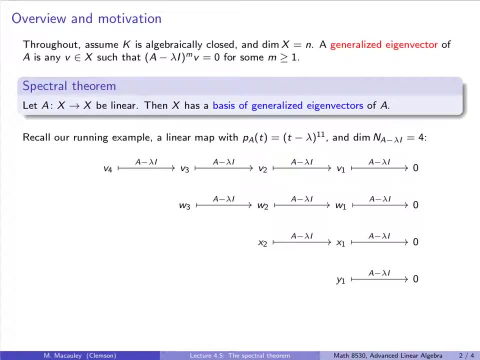 so we can pull this back and get a v4 and a v5 and now we have 11 linearly independent vectors and hence a basis of our underlying space, x. if we let nj denote the null space of a minus lambda i to the j, and it's easy to see that if i 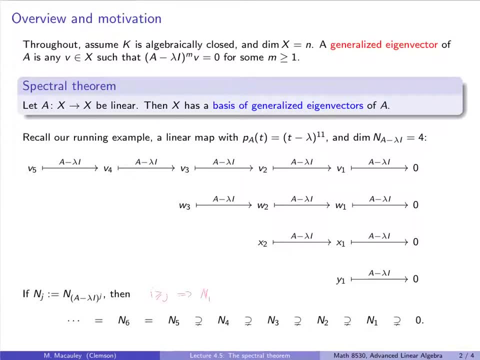 is at least as big as j, then the null space of i is going to contain the null space of i and it's going to contain the null space of i space of j. So we always have this increasing sequence of subspaces Up here. n1 is the 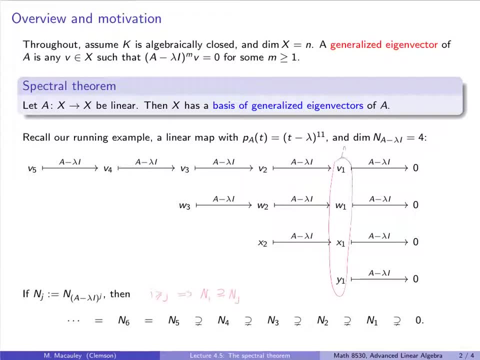 span of the eigenvectors, So this is n1.. n2 is the span of these seven vectors, So this is four-dimensional. This is seven-dimensional. n3 is going to be nine-dimensional, n4,, 10.. And n5,. 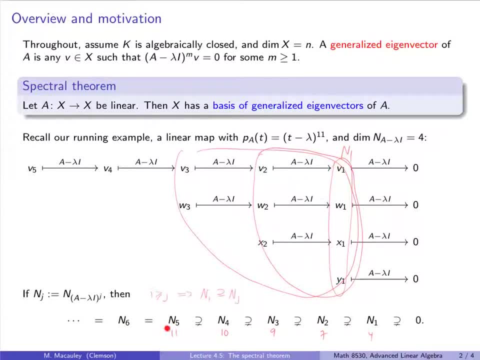 11-dimensional, And then it stabilizes: n6 is equal to n5, and so forth. So notice that, for example, n3 is the set of all vectors, such that if you apply a minus lambda i three times, it gets sent to zero. So what we will do in this lecture is we will define 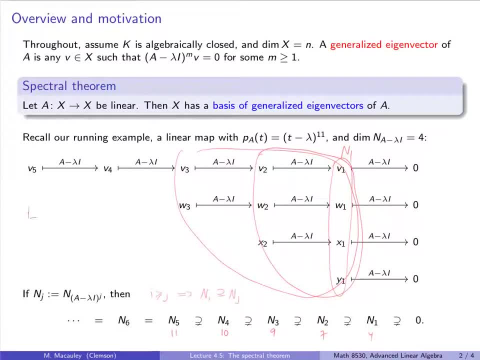 the eigenspace of lambda. so e lambda to be basically all of these things. So one way to write that is: it's the union from j equals one to infinity of nj. So obviously this is in this case equal to j equals one up to five of nj, because we don't ever get anything by going beyond five. 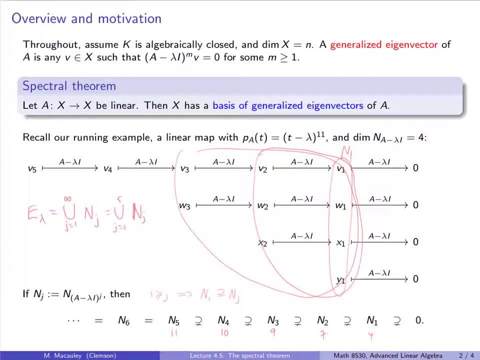 So the spectral theorem where we are going with this is we can always write x as a direct sum of eigenspaces in this manner, or I call them generalized, So lambda, or e lambda one up to e lambda k, where these are the distinct eigenvalues. 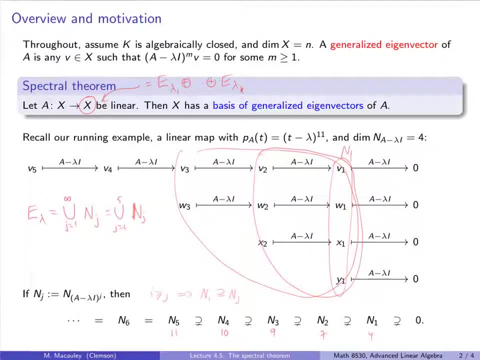 Now we won't be able to prove everything about this picture in this lecture. What we will prove is that for each lambda there is a basis of eigenvectors like this. What we won't be able to prove just yet is that these eigenvectors come in these so-called chains, For example. 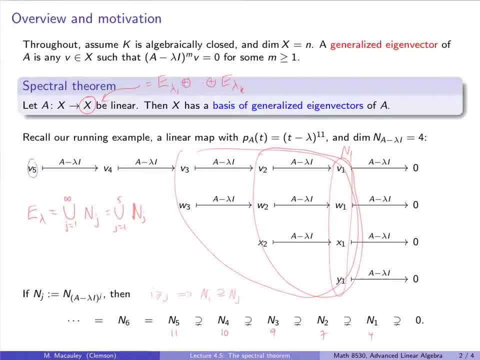 it's not. it's going to be clear why there has to be an fv5 here. Why can there not be a v4 prime that also gets mapped to v3? And in fact there will be other vectors that get mapped to v3,. 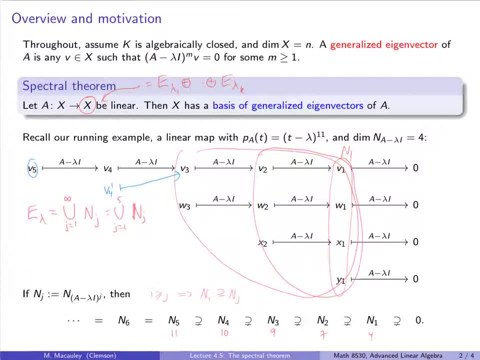 but these will be equivalent in some quotient space. So again, we will show that for any lambda there is going to be a basis of generalized eigenvectors of- we'll call that e lambda, And the dimension of this is going to be equal to the algebraic multiplicity. 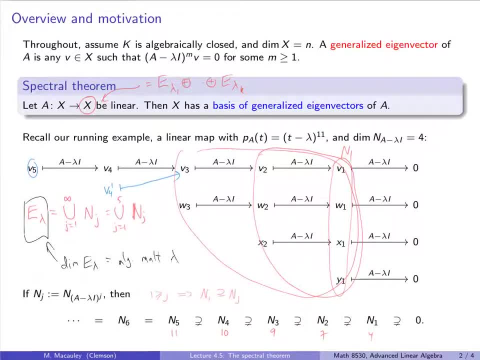 of lambda, which is the degree of t minus lambda, which is the degree of t minus lambda in the characteristic polynomial. And then, in the following lecture, we will actually construct this basis and show that they have to come in this way. So we will show that there is a basis of 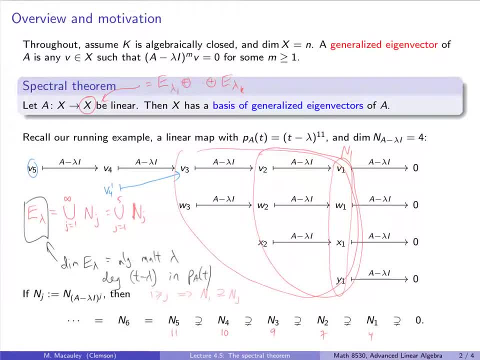 generalized eigenvectors of lambda. this eigenvector of lambda, this e lambda of lambda, is the degree of t minus lambda, and this is the degree of t minus lambda, And we can very clearlyперve schreiben从 Cette веч confidently. 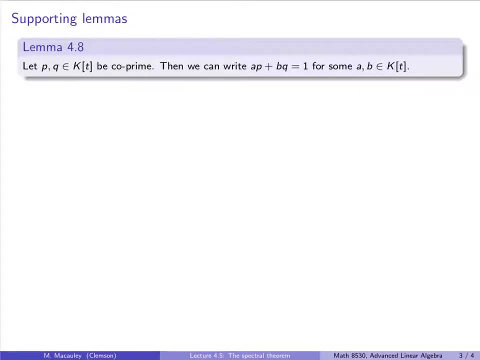 Our first task at hand involves polynomials Over a field, and it basically just follows from the division algorithm and the fact that k of t is a Euclidean domain. So let's let p and q be polynomials shirt over k that are co-prime, Since k is a field. this is equivalent to saying that: 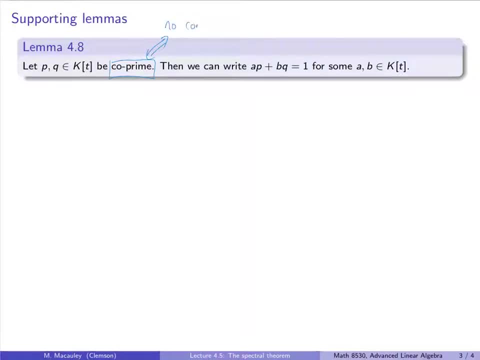 p and q have no common roots, Then I claim that we can write a p plus b q to get 1 for some polynomials a and b. Let's compare this to the integers. A basic fact from number theory, or likely just your intro to proofs class, says that: 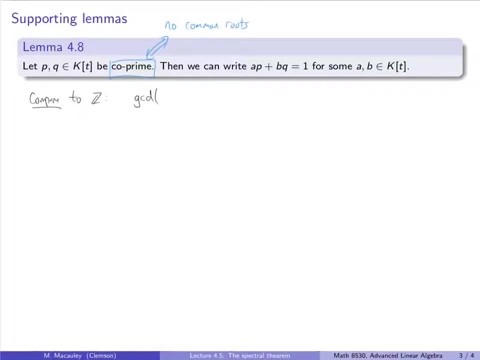 if the GCD of, say, x and y is some, let's call it d, then we can write ax plus by equals d. In fact, d is the smallest positive integer that we can do this for. for for some integers. 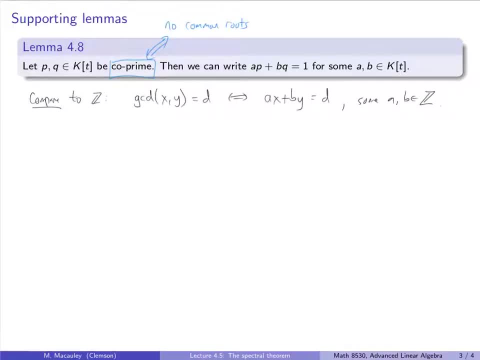 a and b, and this holds because the- the integers- is a Euclidean domain, which means basically the Euclidean algorithm, the division algorithm, work, and so is this ring. now recall what the division algorithm tells us: over z, it means that we can write. I'm so given me say this by given. 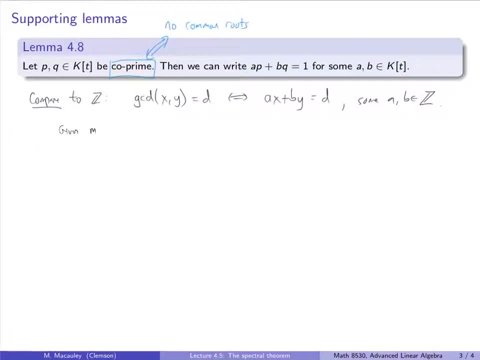 M and are actually happen. if I say, given n and D or D is non-zero, we can write or we can divide D into n and get n equals Q, D plus are and ours the remainder, which is between 0 and D. so could be 0, but it's strictly less than D. so for 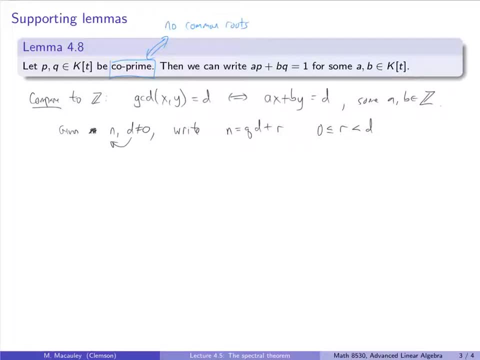 for polynomials, we can do the same thing, but now are are norm instead of being just the absolute value is going to be that agree. so in other words, over over K, T, we can write I'm and love, T equals. so we have polynomials, and D so we can divide. 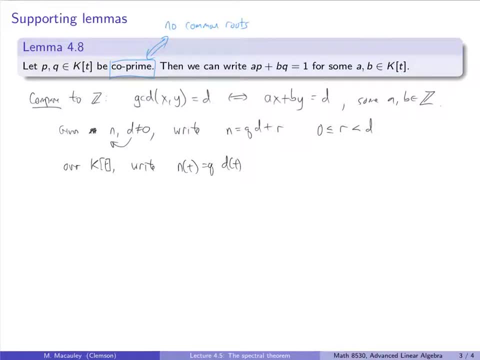 D into n. the event times Q of T plus are: have T where the did. I should say that the degree %uh are is less than the degree up to this little bit, a background that I know I repeated a previous lecture. but let's, let's go with it. 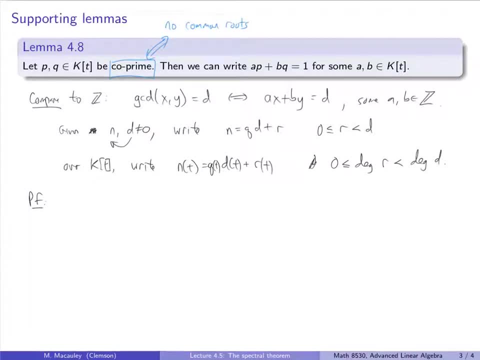 so let's actually do the a, the proof it is now. this should remind you of what we did think in the previous lecture, where I'm gonna let a I be the set up, all things. I can write up this form: AP plus be cute, so a P plus be. 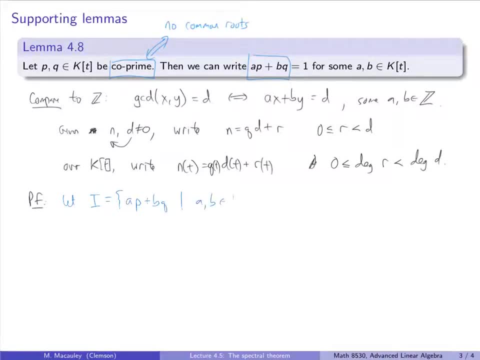 Q, where a and B are polynomials over K it. now all you show is that this contains one, or actually this contains any non-zero constant, because were over a field, so if I have something that's not zero, I could just scale to get one. okay, so this? 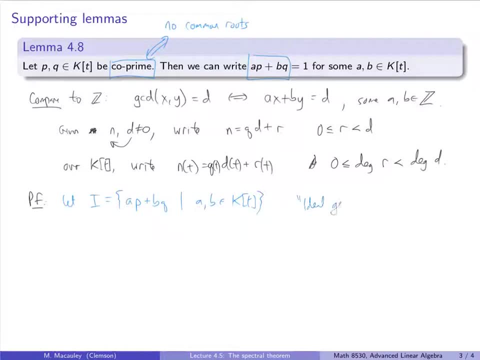 is technically the ideal generated by p and Q. and if you don't remember, knower, remember when an ideal is in ring theory, that's fine. just know that it's all linear combinations. so it's closed under addition, subtraction and multiplication by any polynomial. so what we'll do now is: let's, let's. 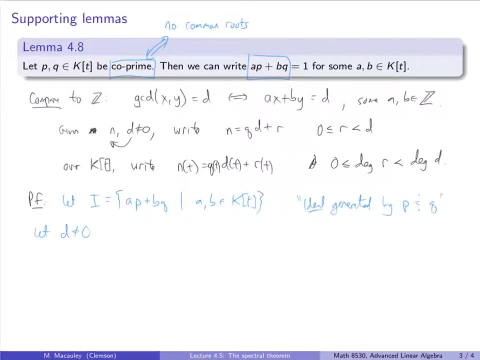 D be the non-zero element in I of minimal degree, Or D is any, because up to scalars, right. So D is an element of I of minimal degree And we're going to. and well, I claim that D divides P and D divides Q. 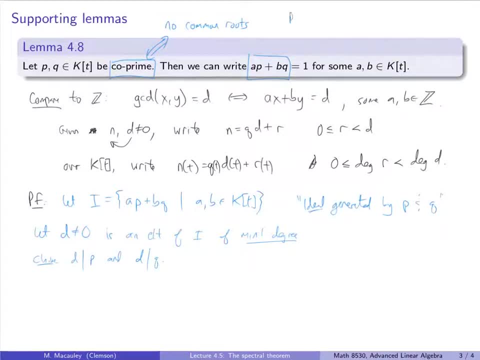 And because there are no common roots if P equals some. so let's write out the roots of P. I don't know if I need to really do this, but why not? Let's say lambda 1 up to lambda m, n and say that Q of T is D. 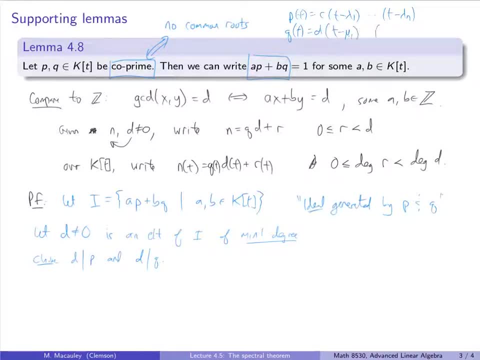 Times T minus mu 1 up to T minus mu m, and these are all distinct. If we have a polynomial that divides both of these, that polynomial has to be constant. So this is all that we have to, so this. so this is all that we need to show. 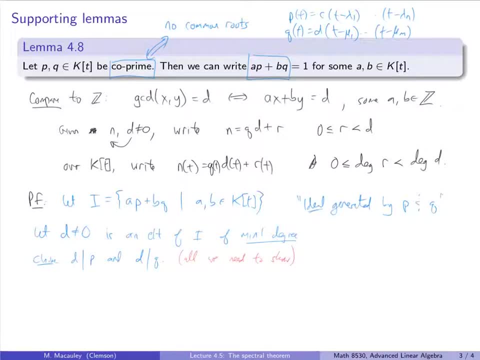 And then we're done. And now there's nothing special about P and Q. They're both, you know, by symmetry. I just need to show that D divides one of them And then, by the same argument, it will divide the other. 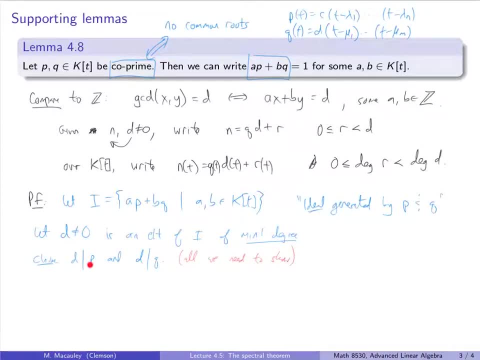 So let's take P and let's show that D divides P. So we will use the division algorithm and we will write: P equals some quotient. Now I've used Q, so I need to use some other letter. Let me use G times P plus R. 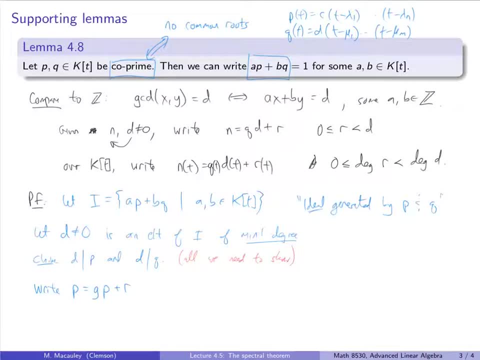 G looks like a Q, but the tail just goes the other way And the degree of R is less than the degree of of D. Oh sorry, I um let me. this has to be a D, not a, not a P. 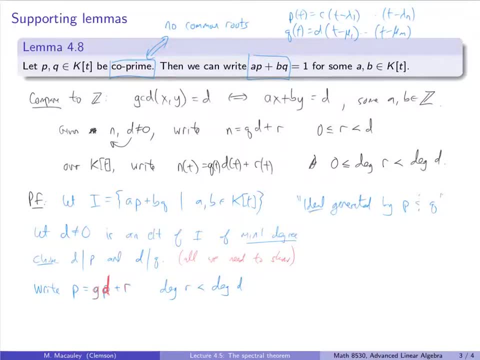 So GD plus R, And now I will solve for R. This is what I did in the previous lecture, So we can write: R equals P minus GD. So now we have a polynomial that has degree strictly less than D, and D had minimal degree. 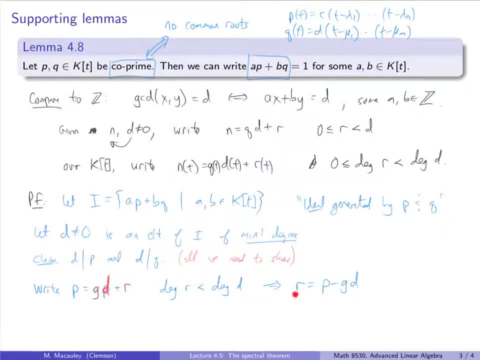 For non-zero polynomials. Now, that's not a contradiction, though. that tells us that R has to be zero. So that tells us that R equals zero. And now we come back here, and if R is zero, that means that P equals GD. 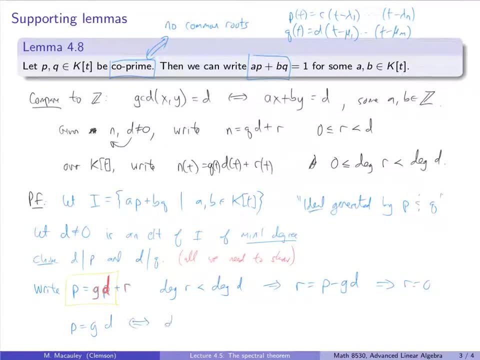 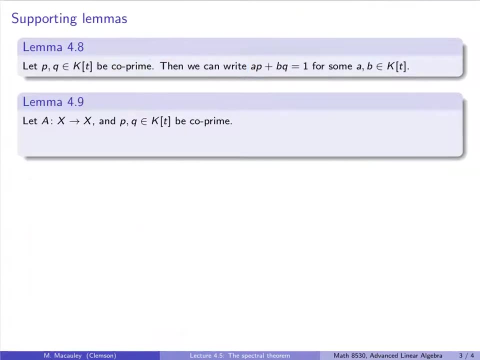 Or in other words, that same thing as saying D divides P, And that is all that we needed to show For our next lemma. let's continue with polynomials P and Q that are co-prime and a linear map A from X to itself. 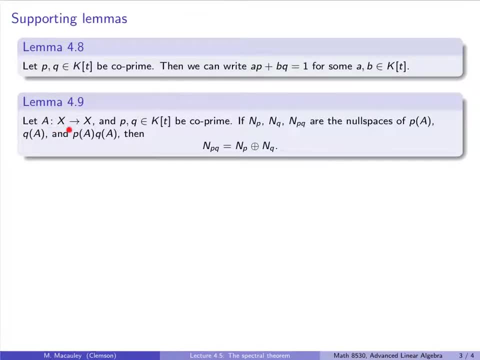 For our next lemma, let's take a linear map A and co-prime polynomials P and Q. just like up here, There are three natural null spaces to look at. We can look at the null space of PA, of Q of A and P of A times Q of A. 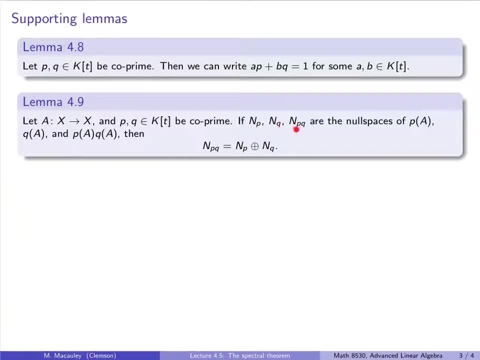 which we will denote by NP, NQ and NPQ respectively. Then what this is saying is that the null space of P, of A, Q of A is the direct sum of NP and NQ. Before we prove this, let's get a little bit more intuition. 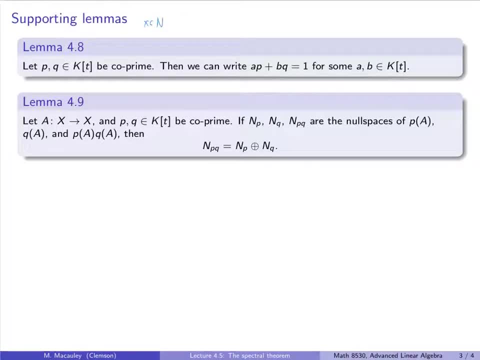 So X is in the null space of P. What does that mean? That means that P of A times X equals zero, X is in the null space of Q, If, and only if, Q of A times X equals zero And X is in the null space of PQ. 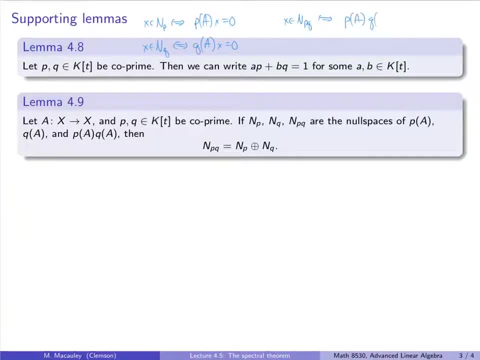 If, and only if, P of A, Q of A, X equals zero. Now, because these are polynomials, in A they commute, So that's the same thing as saying Q of A times P of A times X equals zero. So notice if X is killed by: 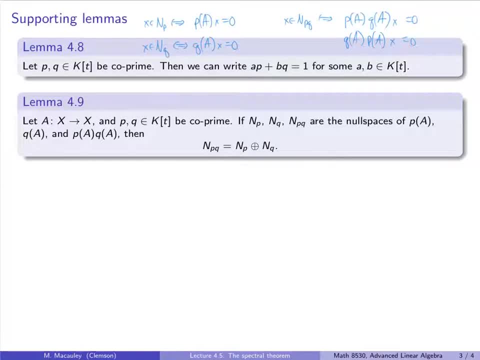 P of A, then clearly X is going to be killed by Q of A P of A, Because that is going to be zero. Similarly, if X is killed by Q of A, then it's clearly killed by it's in NPQ as well. 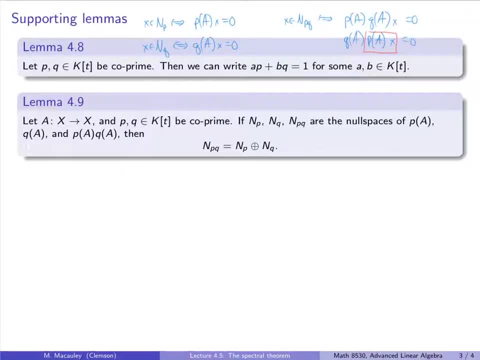 Because Q of A X is equal to zero. So this whole polynomial times X will be zero. So, in other words, this tells us, this shows right away that NP is contained in NPQ And also NQ is contained in that as well. 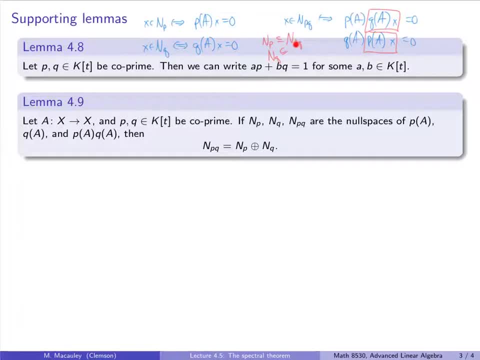 So what I claim is that this is everything in here- can be represented uniquely. In other words, every vector that's killed by P of A times Q of A is killed by either P of A or Q of A, So there's nothing else in between. 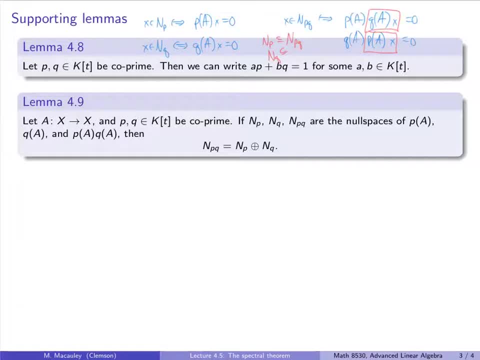 So that's one thing that I claim. So let me write that down Like. my first claim is that everything in P? Q can be represented as NP, as something killed by P and something killed. everything in NPQ can be represented as: 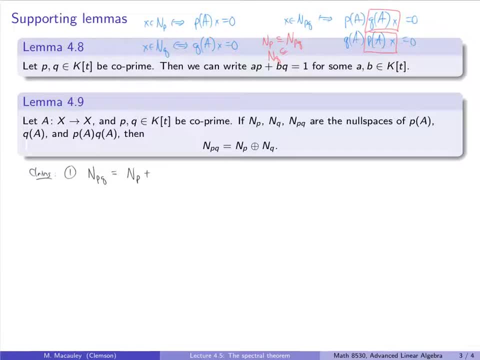 the sum of something in NP plus something in NQ. In other words: yeah, I argued that out here, Let's keep going. So this just says that NPQ is the sum of these two subspaces, And remember what it means. 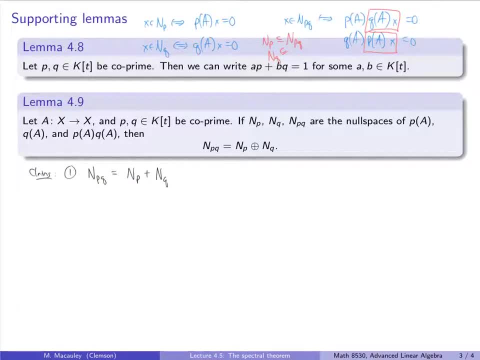 for this to be the direct sum. Well, that means that first of all it has to be the sum, but also these are complementary subspaces, So they intersect trivially in the zero vector. Now another equivalent way to say that: 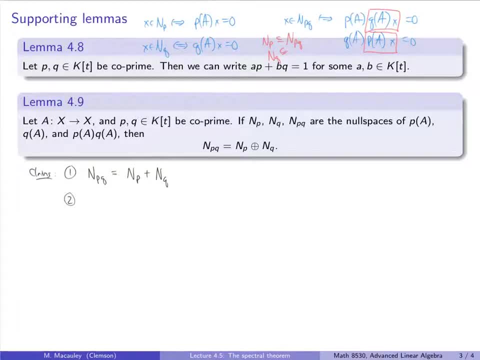 this is a direct sum, is that everything in here can be written as a sum of something in here and something in here uniquely? So let's let me say that So X, everything in NP can be represented as something I'll say as a sum of XP plus XQ. 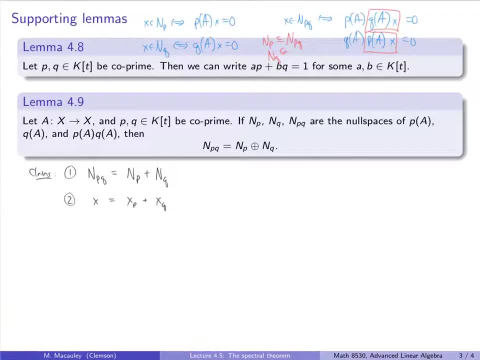 where XP is in NP, XQ is in NQ. Well, this we get from the previous part, but what's new here is this uniquely part. So this, this decomposition is unique, So we will show these one by one. 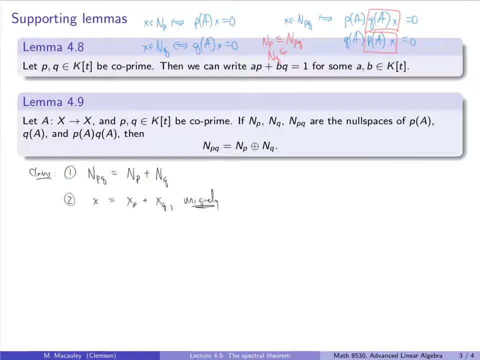 So first let's show that NPQ is the sum of these two vector spaces, And to do that, what we will do is use this lemma And we will write one as AP plus BQ, And then we will analyze that. 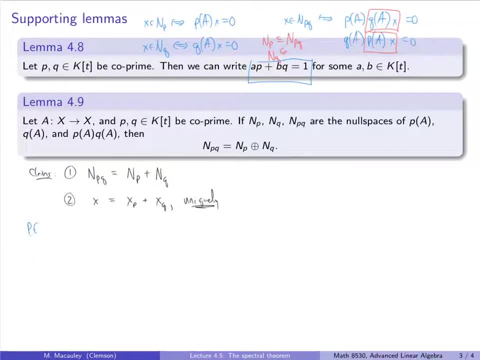 So let's do that first. So let's, so let's write A of T, B of T plus B of T, Q of T, equaling one for sum A and B. We know we can do that, And now, what we will do is we will plug in A. 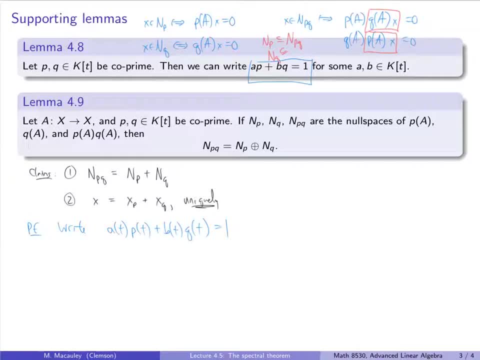 And the right-hand side, we will get the identity matrix. And the left-hand side- we're going to get something that we claim is is not going to be the identity. So let's, let's do that and see what happens. 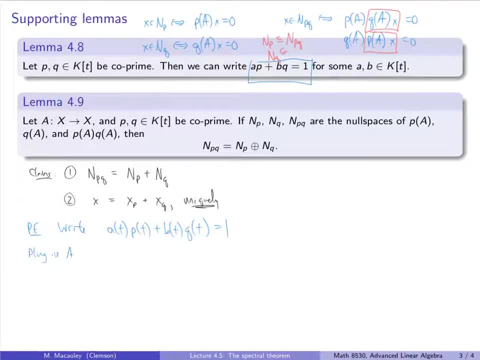 So let's plug, plug in A And we get A of big A, P of big A plus B of big A. Q times big A equals the identity. And now we will take this and we will multiply this to by on the right. 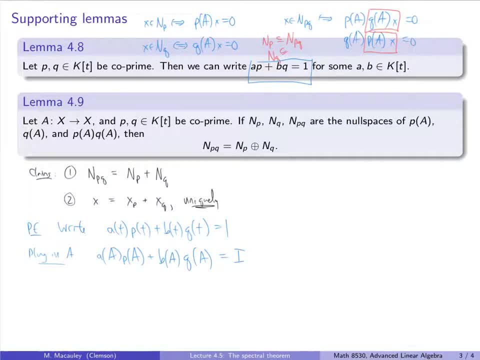 by a vector in A And PQ. So let's, let's multiply by some X in N- PQ, And if we do this we get A of A P of A X. let me do this in red so you can see it. 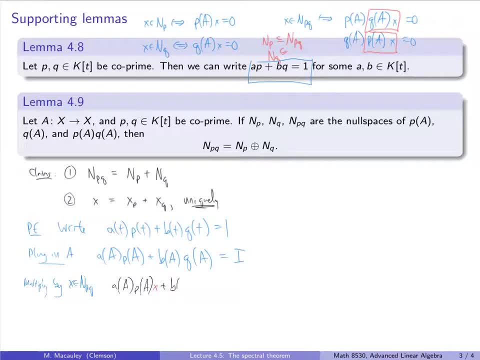 X plus B of A, Q of A. X equals I times X, which equals X. So I have just taken an arbitrary element in N P Q and I claim that what I have done is I have written it as a sum of something in N P. 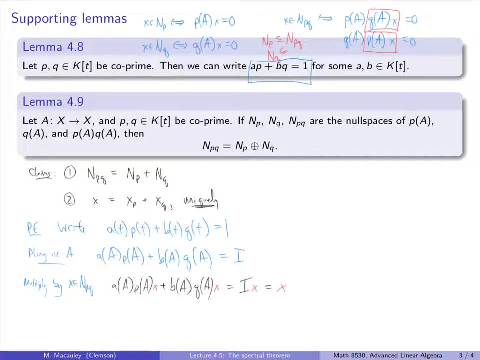 and something in N Q. And to see why that is, let's look at this P of A times X and this Q of A times X. So because X is in N P Q, that means that by definition, P of A, 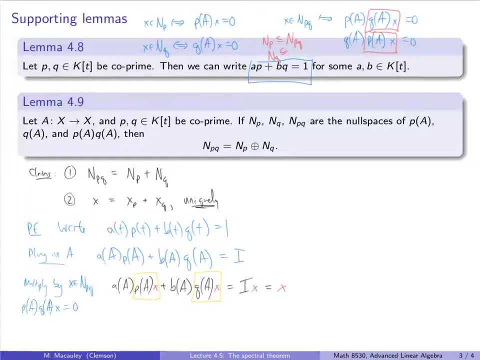 Q of A- X equals zero. or, equivalently, Q of A- P of A- X equals zero. So notice that this entire first term if I multiply it on the left by Q of A. so let's think about what happens. 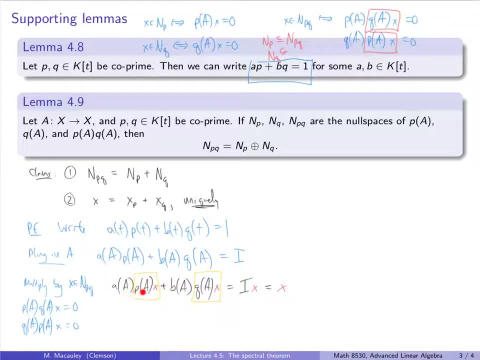 if you multiply this by Q of A, Now these polynomials commute because they are polynomials in A. So if I multiply by Q of A, we get P of A, Q of A times X, and that's zero. So in other words, 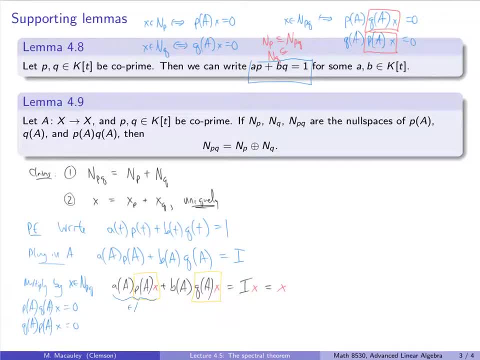 this entire term here is in N Q. It's killed by Q of A. Similarly, this entire term here is killed by P of A. If I multiply on the left by P of A, I get P of A times Q of A times X. 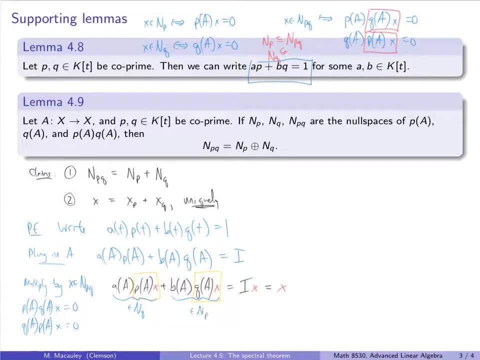 So this is in N P. I have just taken my an arbitrary element and written it as something in N P and something in N Q. So that confirms part one. Now for part two. How do we show uniqueness? Well, let's. 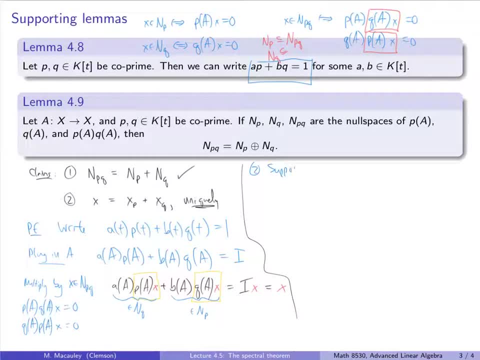 let's suppose that there's two ways to write X. Let's write that as a. let's say that X equals X P plus X Q, and also X prime P plus X prime Q, where I'm just going to say it. 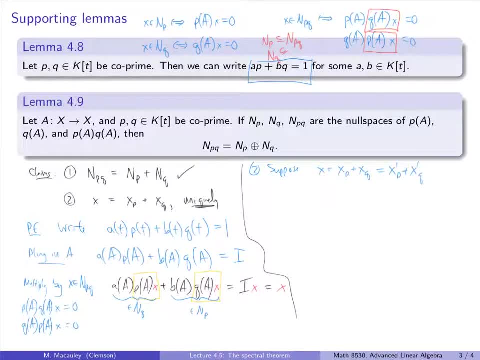 I'm not going to write it. X P and X P prime are in N P and X Q and X Q prime are in N Q. So we'll take this and we'll move all the X, both the X P's, to the left. 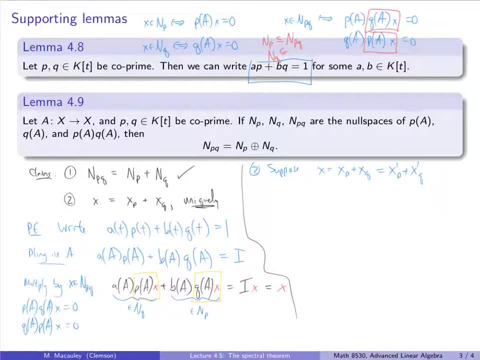 same side and the X Q's to the other side. So in other words, we get X P minus X prime P equals X Q prime or X prime Q, however you want to say it, minus X Q. Now this. 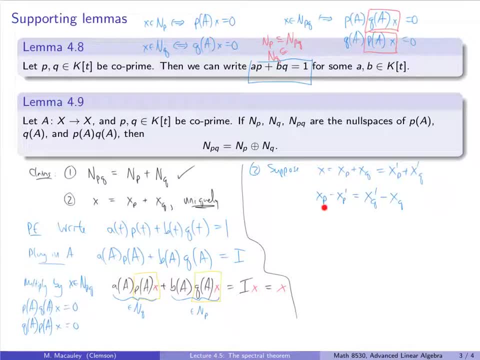 because these are subspaces. this is in N P and in N Q. So I, this is in N P and N Q. Now, remember to show that this is a direct sum, we have to show that this is precisely the zero vector. 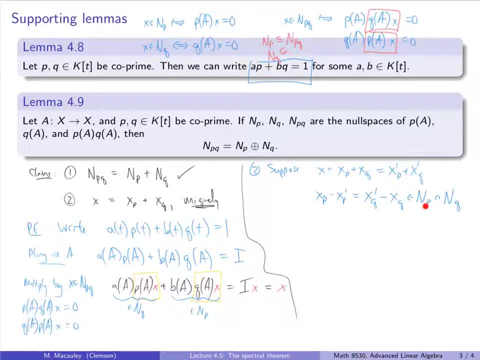 They intersect trivially, Okay, so? so how do we do that? Well, first of all, let's give this thing a name. Let's call this Z, because we want to show it is zero. And what I will do is: 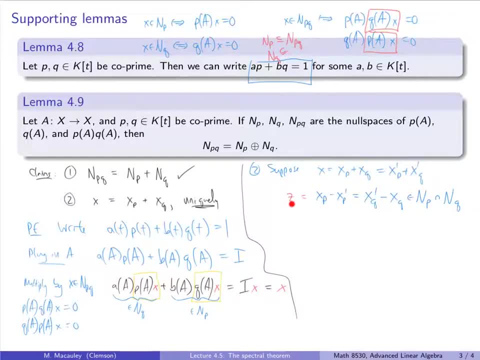 I will show that this is zero by taking Z and multiplying it by the identity matrix, which we know is A. is this expression right here? A of A, P of A plus B of A, Q of A? If I can show that Z is killed by this expression, 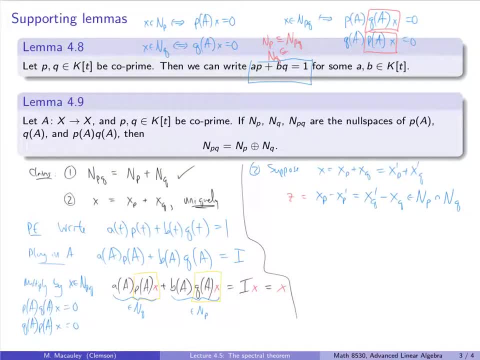 which is the identity matrix, then Z has to be zero. Okay, so how do I want to write that down? So multiply by. I let me box it. so I'm going to multiply this by this. I So A of A, P of A. 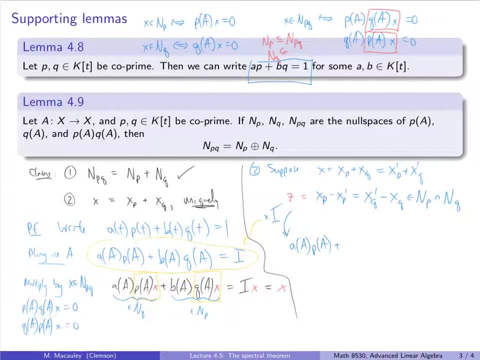 times. well, let's do first B of A, Q of A. this entire thing: times Z equals I, Z equals Z. So what happens here? Let's break this into two parts: A of A, P of A times Z plus B of A. 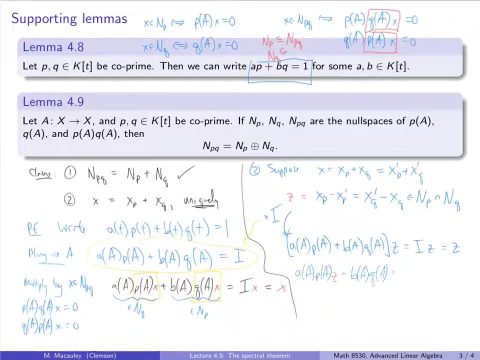 Q of A times Z. Now remember, Z is killed or Z is in both of these. so Z is killed by P of A and by Q of A. So that must be zero, and that must be zero. So therefore, 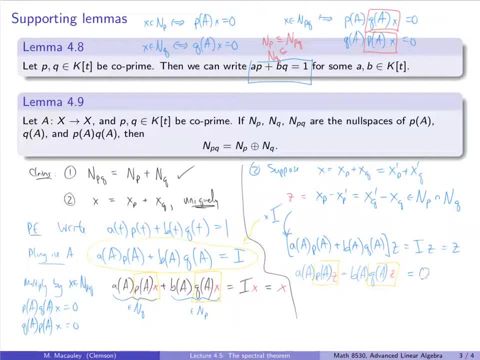 this is equal to zero. So we have just- I've just showed you that- an arbitrary element. or well, let's see what have I showed you? I've showed you that this decomposition is unique because the difference Z has to be zero. 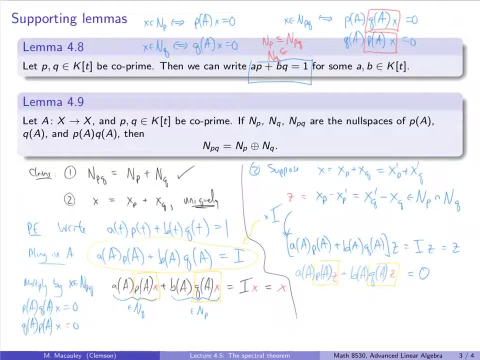 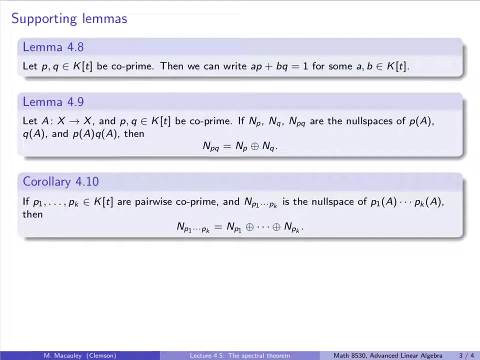 And that's how we establish uniqueness and how we establish that this is a direct sum. It is straightforward to extend lemma 4.9 from two polynomials to K polynomials. I won't even bother reading this thing. I think it's easy enough. 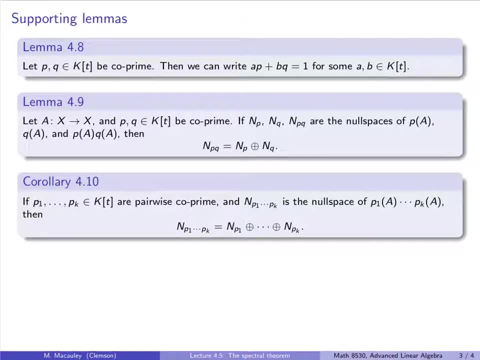 to look at and see that it's true, And let's talk about why we care to do this. So let's let P of T be the characteristic polynomial of A, So we can write P of T as T minus lambda 1. 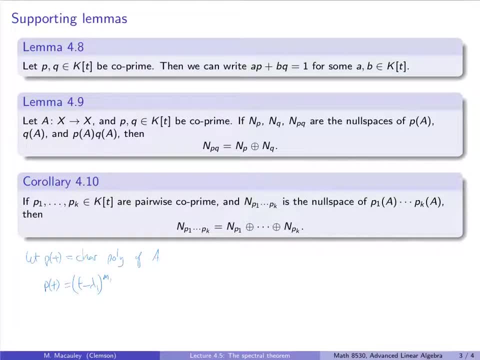 to the, let's say, M1 times T minus lambda 2 to the M2, all the way up to T minus lambda K to the MK, where these are distinct eigenvalues. Now, let's call this P1.. Let's call this P2.. 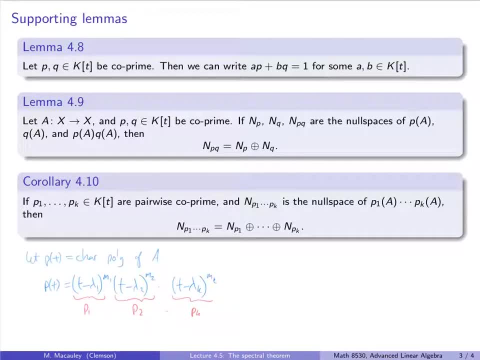 And let's call this PK And think about what happens when we plug in A By the Cayley-Hamilton theorem: P of A is the zero map. So the null space of P of A, the null space of the zero map. 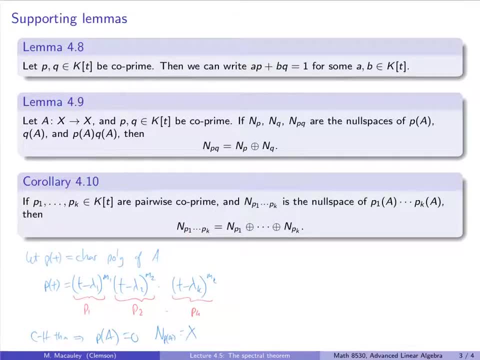 is everything. So in this case this space, N sub P1 up to PK, is equal to X. So that means that everything in X can be represented uniquely as a sum of things in these individual NPJs. And think about what that is. 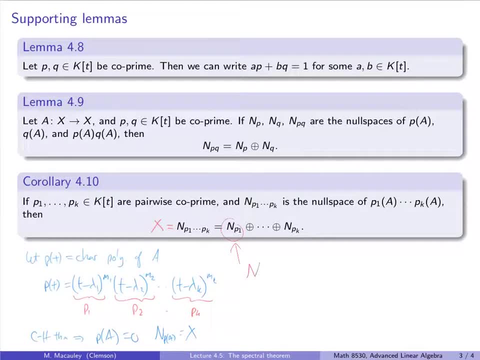 So NP1 is the null space of A minus lambda 1 I to the M1. And so forth. And PK is the null space of A minus lambda K times I to the MK. These are spaces of generalized eigenvectors. This is precisely. 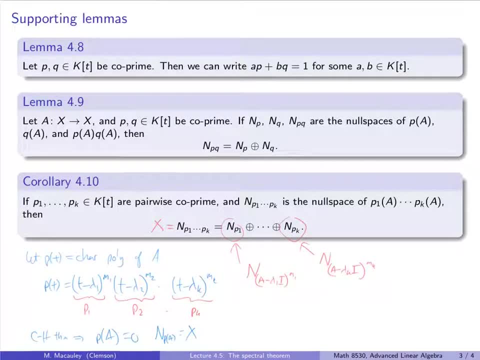 the set of all generalized eigenvectors for lambda 1. And so forth. So everything in X can be represented uniquely as a sum of generalized eigenvectors. So this is the set of generalized eigenvectors for each eigenvalue. 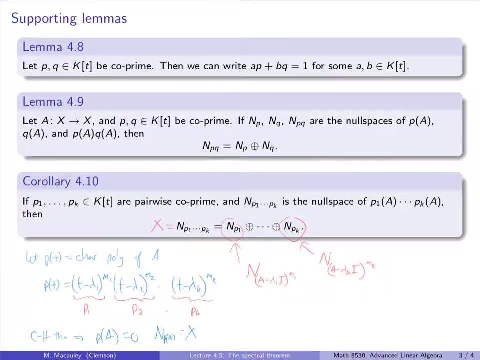 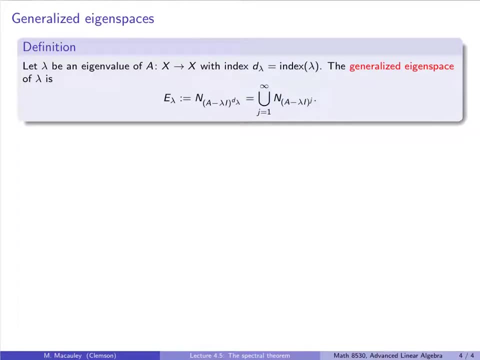 There it is. I've basically proven the Spectral Theorem. I will finish this lecture with a slightly stronger reworded version of the Spectral Theorem that speaks in terms of generalized eigenspaces instead of generalized eigenvectors. So let me remind you. 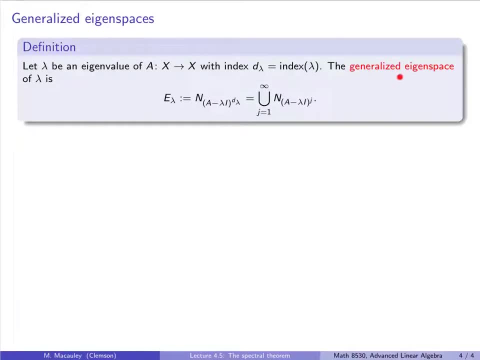 of the definition of a generalized eigenspace. I think I wrote it in the margin on the first slide. So if A is a linear map from X to itself and lambda is an eigenvalue with index d lambda, then the generalized eigenspace. 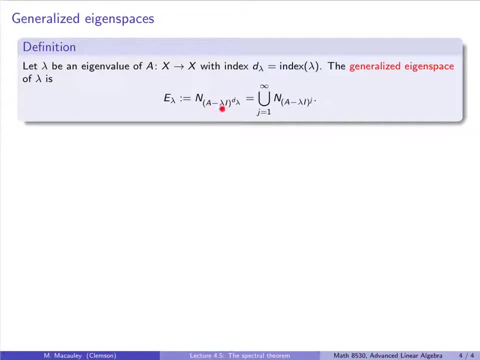 is just the nullspace of A minus lambda I to the d lambda Which, as I said before, is the sum of all A minus lambda I to the j up to from 1 to infinity. that we can really stop at d lambda. 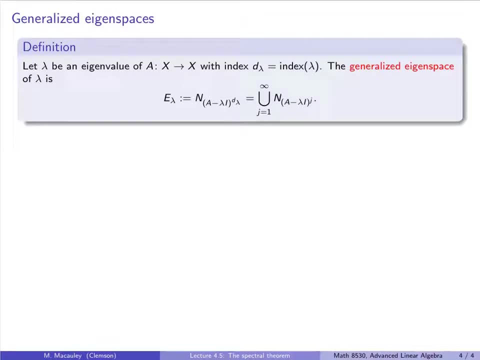 Now, this is still the better definition, because for infinite-dimensional spaces- and I will show you one in a couple of lectures- involving differential operators, sometimes this sequence gets bigger and bigger for all j. So, in other words, this sequence doesn't stabilize. 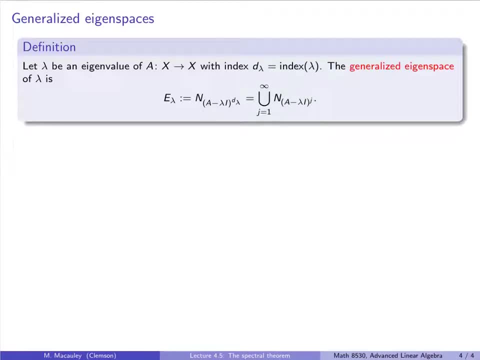 like we saw in our 11-dimensional example. Our strong version of the Spectral Theorem, which is pretty easily seen to be equivalent, is that if we have a linear map with distinct eigenvalues, lambda I up to lambda k, then X is a direct sum. 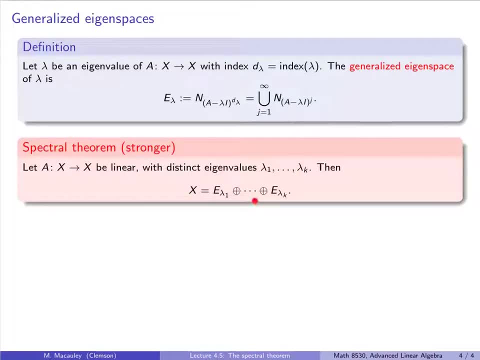 of eigenspaces: e lambda I up to e lambda k. So let's prove this, And we will let P of T be the characteristic polynomial and write P of T. so it's really not much different than what I just did: T minus. 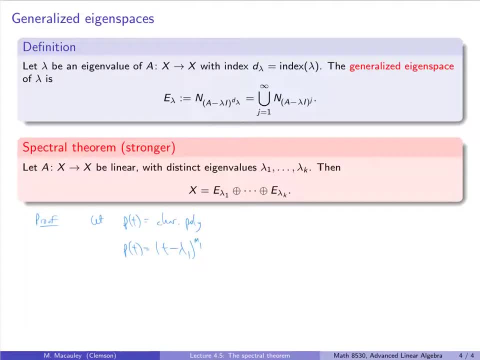 so I'll do it kind of quickly: T minus lambda I to the m1, all the way up to T minus lambda k to the mk, which we'll call P1, up to Pk. Then the null space of P of A, which I've already explained, is X. 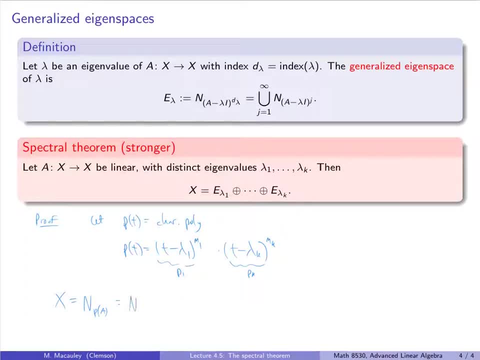 because that's the null space of the zero map, is the null space of P1 of A, the direct sum of this up to the null space of Pk. So this, of course, is the null space of A minus lambda I. 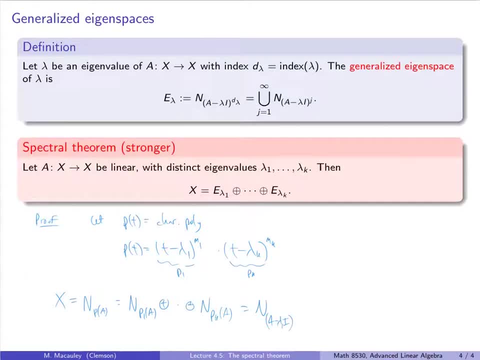 lambda 1: I to the m1, plus dot, dot dot, the null space of A. minus lambda k: I to the mk. So this says that everything in X can be represented uniquely as a sum of generalized eigenvectors for each eigenvalue, In other words: 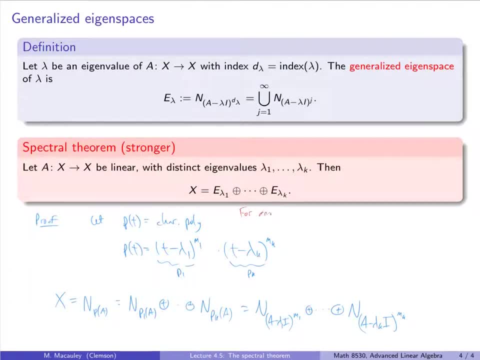 anything, in other words, for any X in X, X equals X1 plus X2 plus all the way up to Xk, where Xj is in the null space of A minus lambda I, lambda j, I to the mj. So these are generalized eigenvectors. 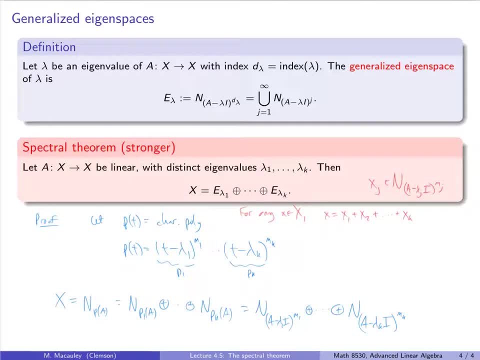 Now I should actually finish with one comment. My original statement of the spectral theorem said there's actually a basis of eigen generalized eigenvectors, And let me write out what that basis is. So if we let B1 be a basis of this, 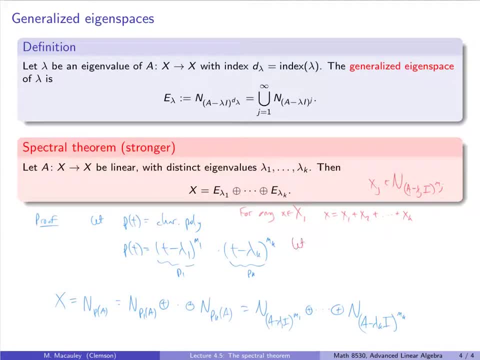 so let's, how about if I write it down like this: Let Bj be any basis of the null space of A minus lambda j, I to the mj, Then I claim that. well, I don't need to claim it, we know that a basis. 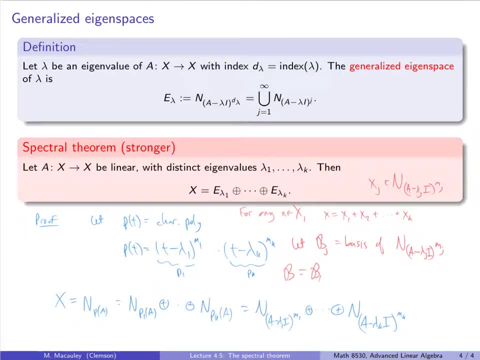 for the direct sum is just a union of the bases, of the individual factors. So B is equal to, so a basis for the direct sum. so a basis for X is just a union of these individual bases And each one of these is. 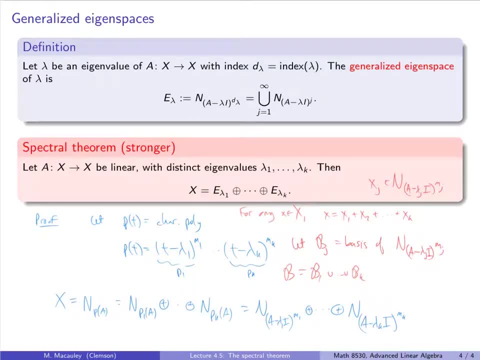 consists of generalized eigenvectors, because each individual space here is a space of generalized eigenvectors. Now, X is not going to be a generalized eigenvector, It's a linear combination of them, But each one of these contains only generalized eigenvectors. 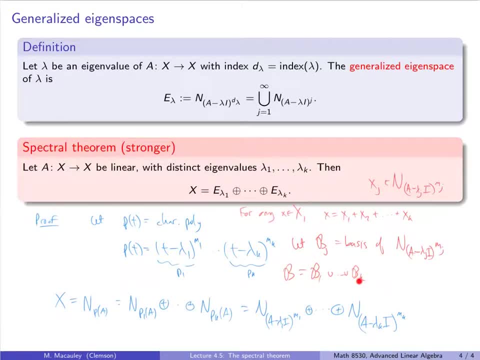 And so, therefore, each basis is only going to contain generalized eigenvectors. So that's actually why my original statement of the spectral theorem is true. Okay, so to summarize, we have now confirmed that X will always have a basis of generalized eigenvectors of A. 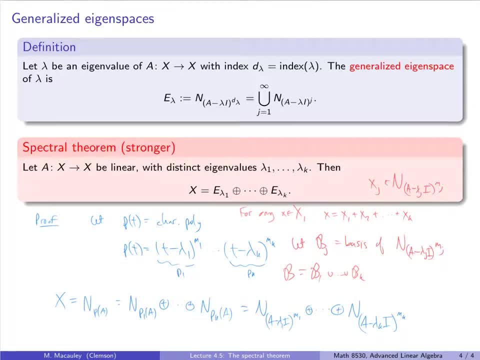 But what we have not yet been able to do is claim why the matrix, with respect to this basis, is going to be the Jordan canonical form. Well, I can't say with respect to any basis, but why we can always find a basis of generalized eigenvectors. 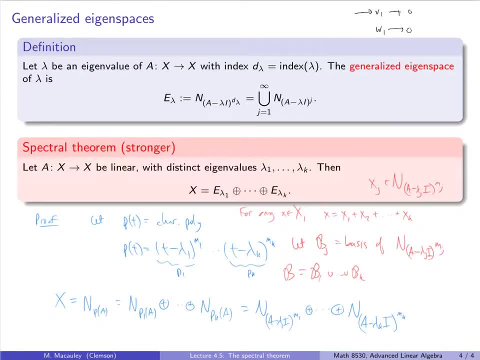 that looks like chains, as I've shown you before. So in other words, what I want to show you is that we can always avoid a case where we have branching like this. So if we do that, then for each lambda we have chains of generalized eigenvectors. 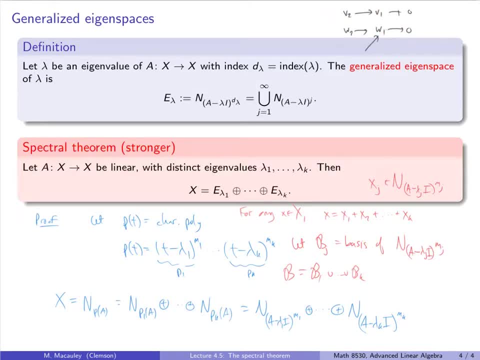 And each one of these chains represents an invariant subspace. So in block diagonal form those are going to be the so-called Jordan blocks. So that will be coming up in the next two lectures. I hope you stick around.